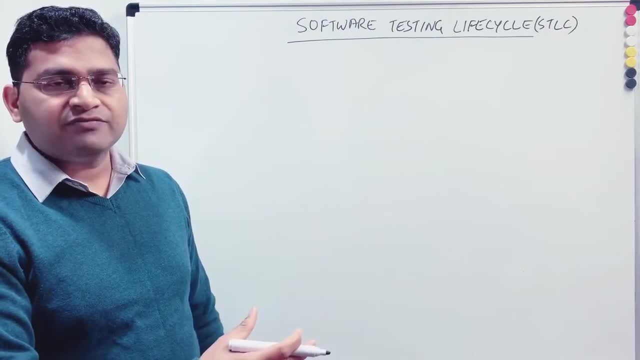 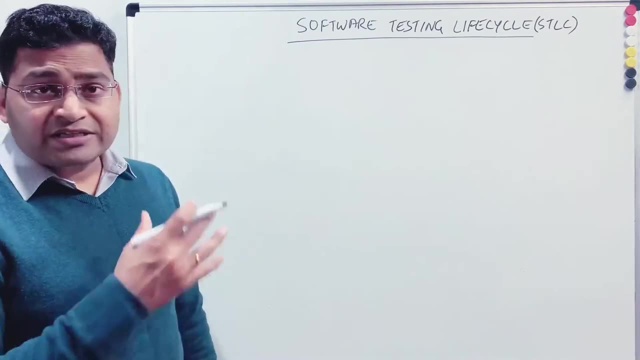 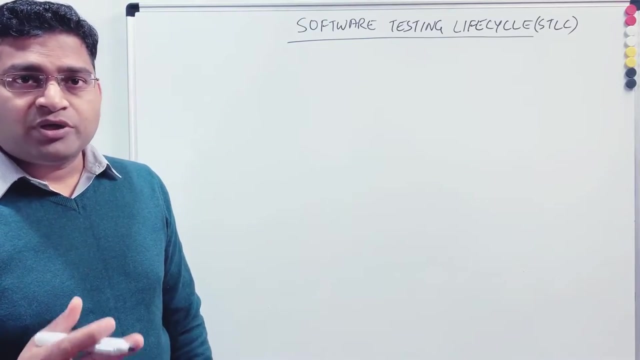 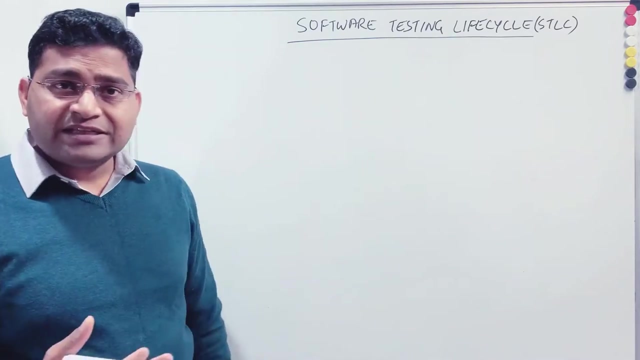 software testing lifecycle fits within the development lifecycle and it is the process of testing any software. So we need to understand software testing lifecycle thoroughly before we can, you know, get into any software testing job. because once you get into the software testing job, or you are trying to get into software testing job, you need to understand how software testing 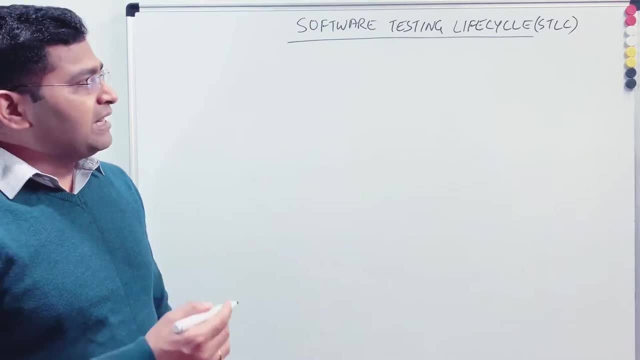 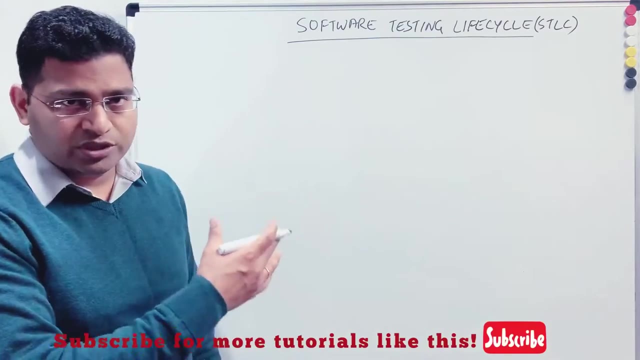 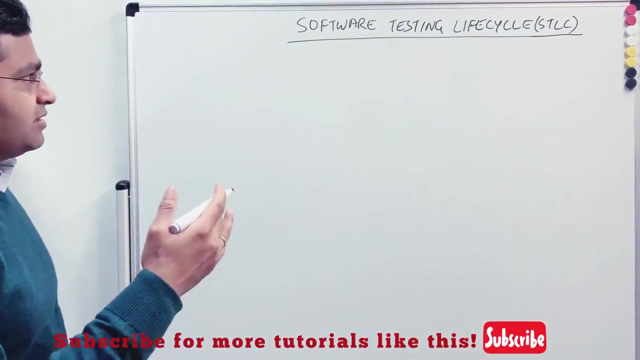 lifecycle, or the process, is actually so that you can, you know, you know the process and you can actually work with the team and come up to speed very quickly when you join any organization. So let's understand what exactly software testing lifecycle is. So it is the set of processes or the phases, basically right. So it's different. 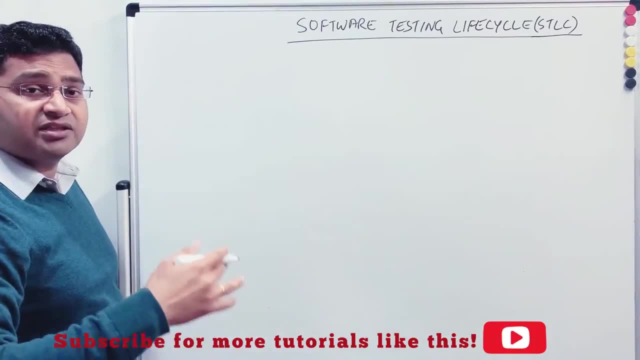 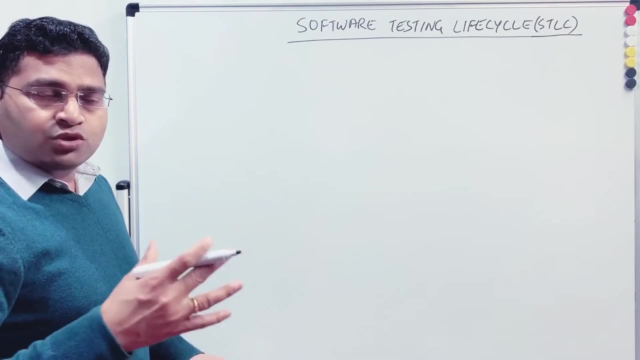 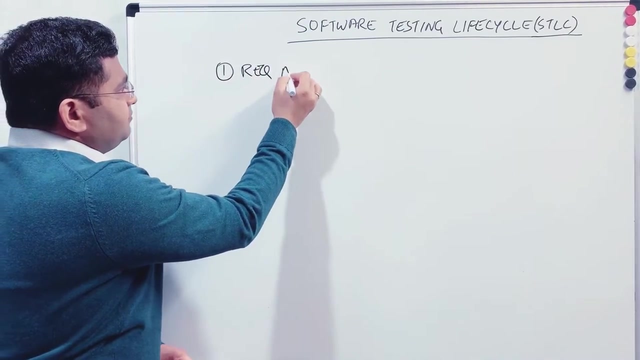 phases are there in software testing lifecycle. The first phase is the requirements analysis. Now, in any software development, the first thing that you will get is the requirements, right? So the first phase in STLC as well, is a requirements analysis. Okay, When we say requirement analysis, 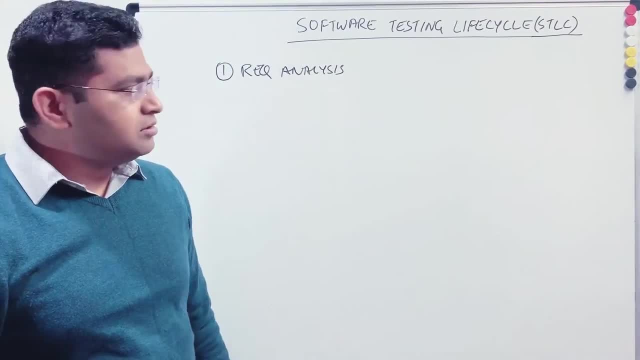 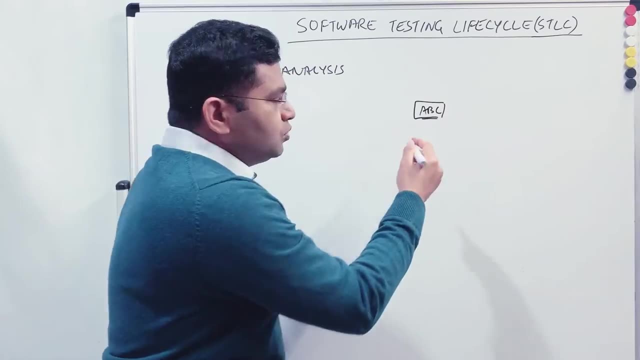 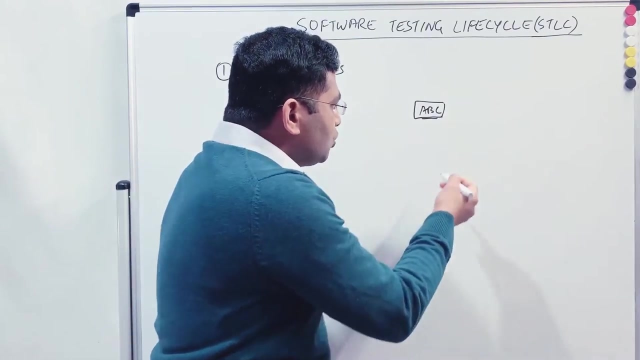 say, for example, I am a software development organization. or say, for example, there is an organization ABC named, which is the organization who takes the project to develop software for the customers. Okay, Now, this organization. how will they? you know? 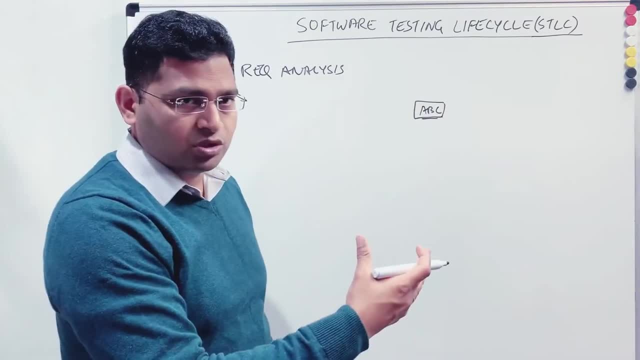 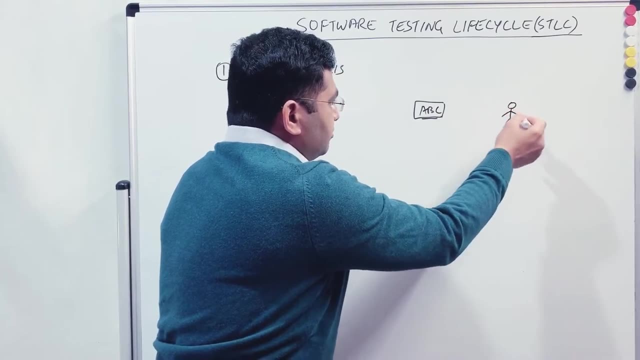 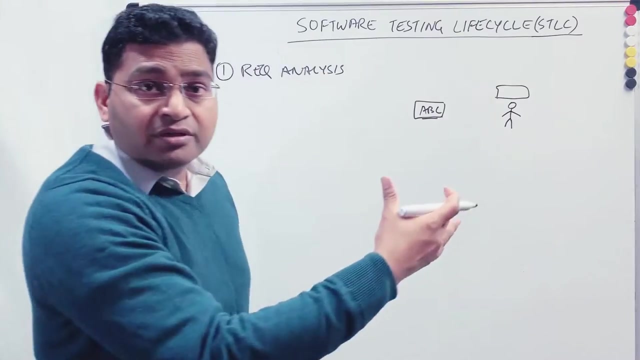 start developing something if they don't know what customer wants, right, So there will be a customer. okay, There will be a customer and the customer- you know, usually it will be organization, right? So I've just made a person there because some person or a group of person, people will be. 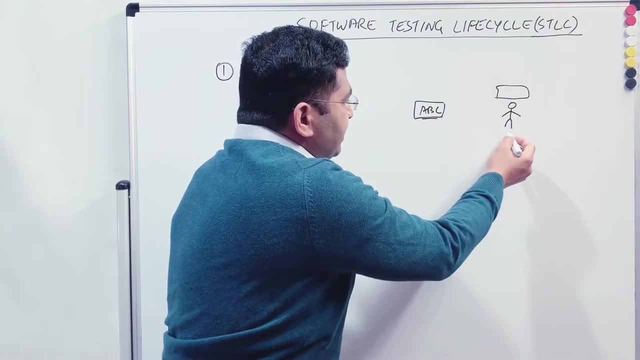 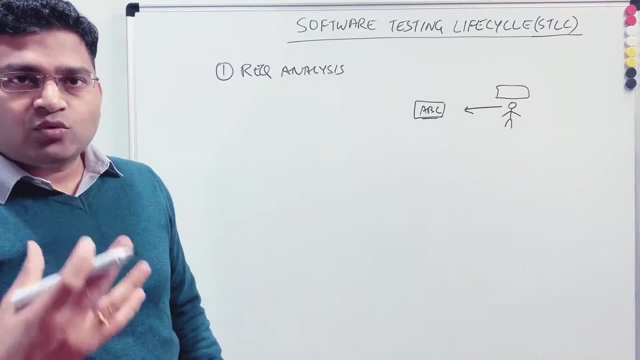 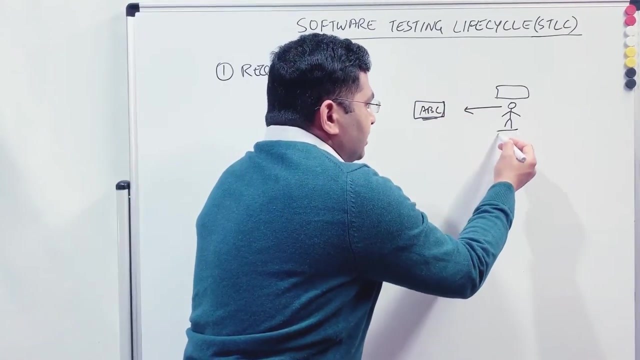 representing that customer organization, and they will come down and they'll, you know, provide or give the requirement, or they will dictate the requirement to this particular ABC organization. Say, for example: this is the organization right, So XYZ is the organization who wants to develop. 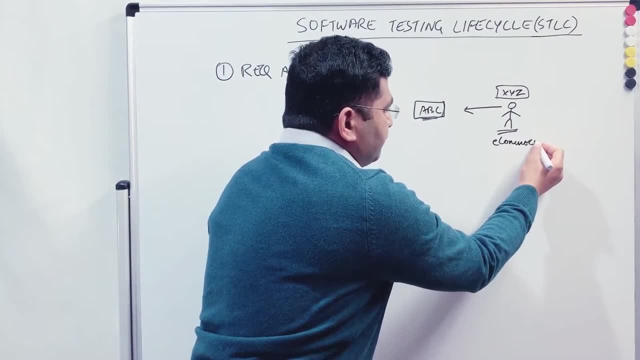 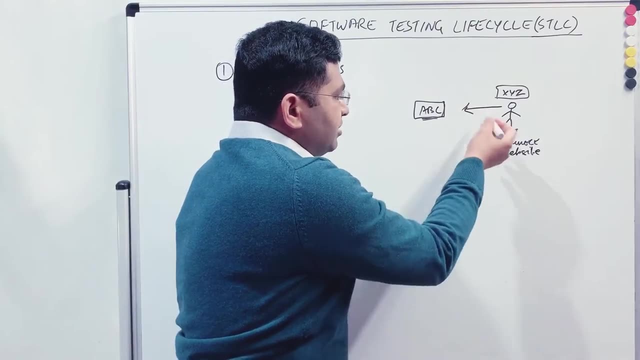 e-commerce. So let's take e-commerce app, e-commerce website. Okay, So what they'll do is they'll come to this particular organization or they'll provide a bid, bidding, and there'll be a couple of organizations that will be bidding. 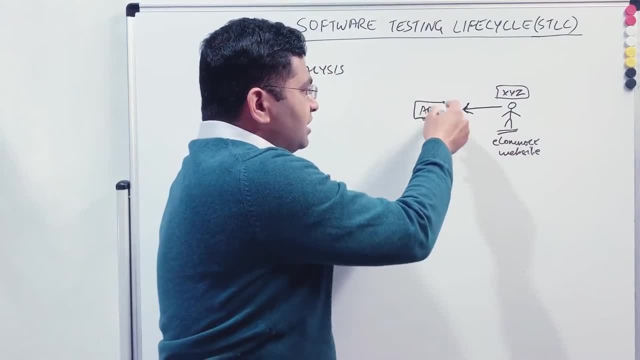 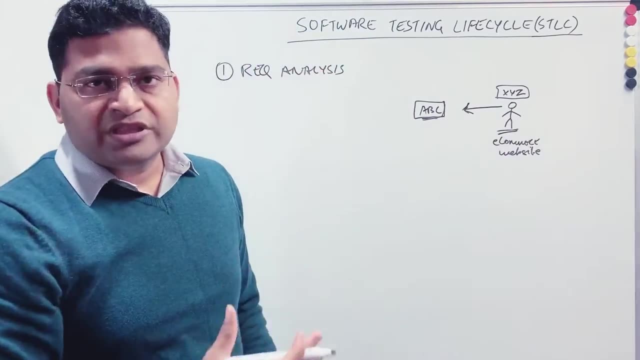 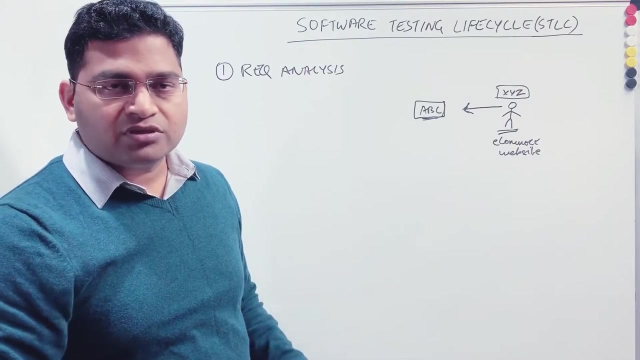 And then, once this organization has won the bid that yes, we'll develop an e-commerce website for you, they'll start explaining what all they want in the e-commerce website. right? So they'll say: we want the website to work on all different browsers- Chrome, Firefox, right, So that's one. 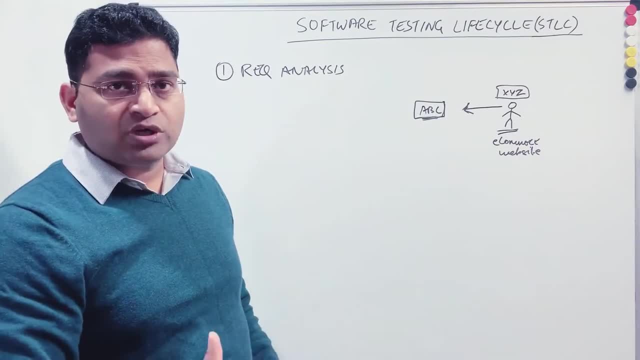 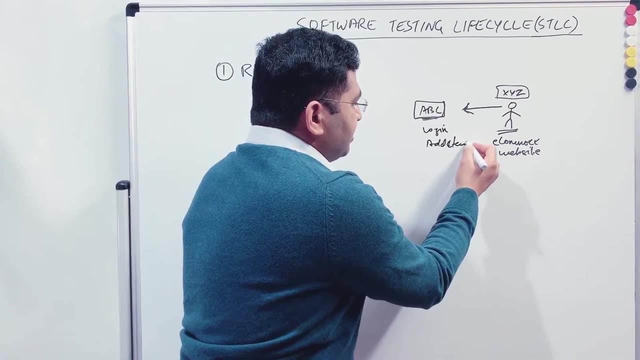 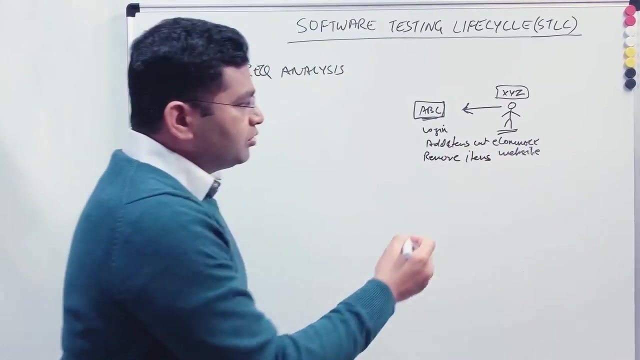 of the requirement: We want the login functionality using Google account, Facebook account, right, So login functionality need to be there. Add add cart. add items to cart. okay, Then remove items to cart. So these are some of the requirement, right, So there'll be. 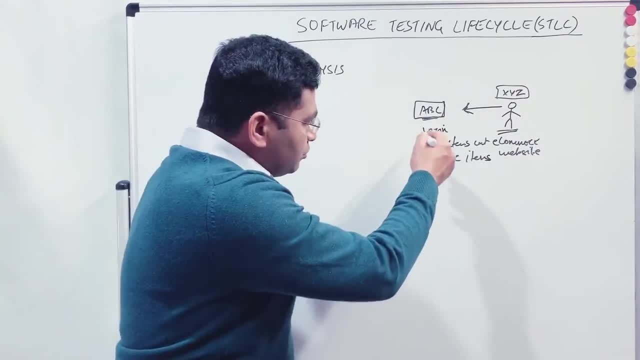 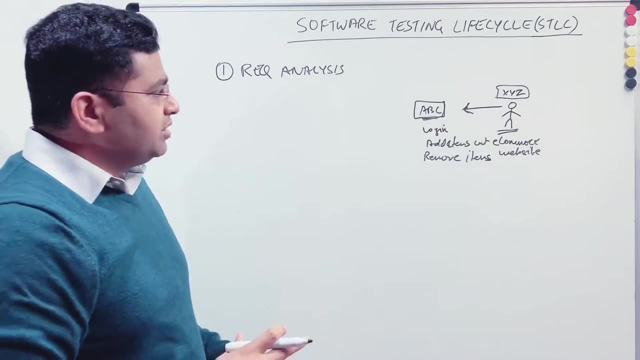 n number of requirement there. So this is just an example. I'm showing you how the requirements will come through. Okay, So once all these requirements are being captured into a document, okay, So if it is waterfall approach, you will be having a lengthy requirements document that. 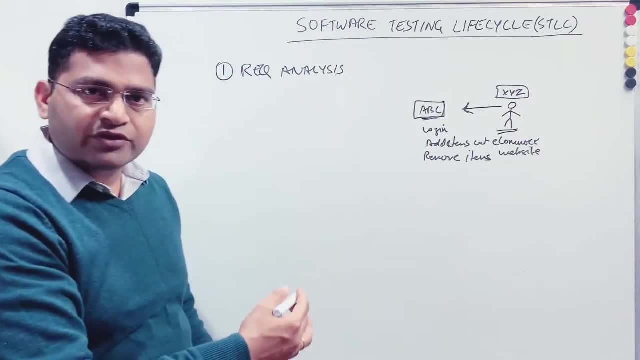 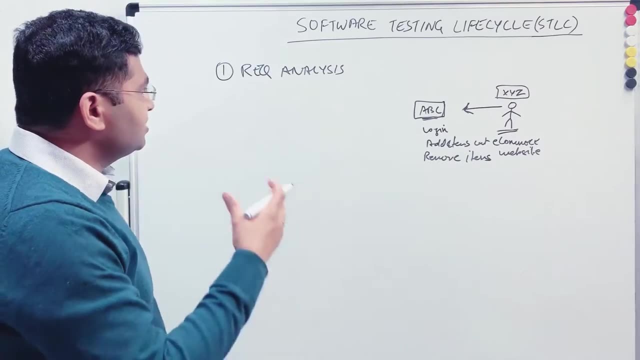 will be catching all these requirements- how the look and feel will be of the website, And those requirements will come through to the ABC organization. There'll be some team in the ABC organization which will start developing the website, Okay, And you as a tester will be. 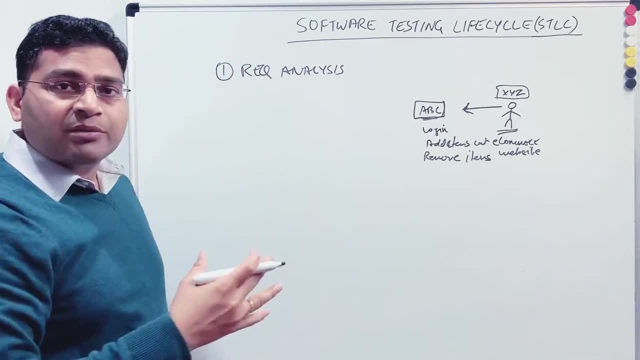 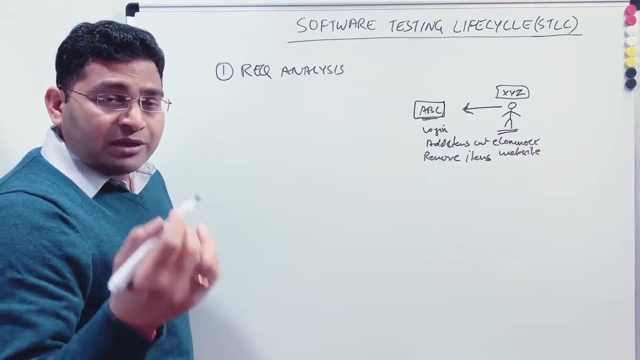 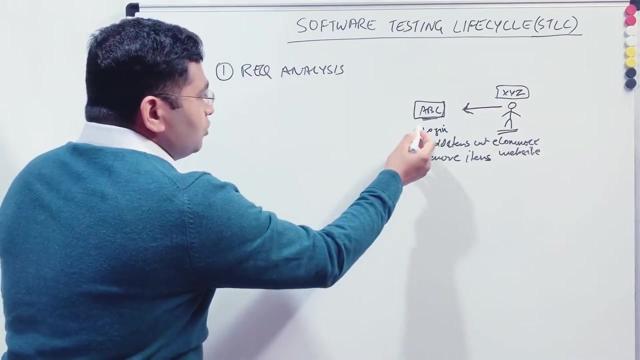 part of that team to basically analyze the requirement and start testing once the website is being built. Okay, So in the requirement analysis, requirement analysis phase of software testing lifecycle, what you do as a tester or a testing team is you get go through these. 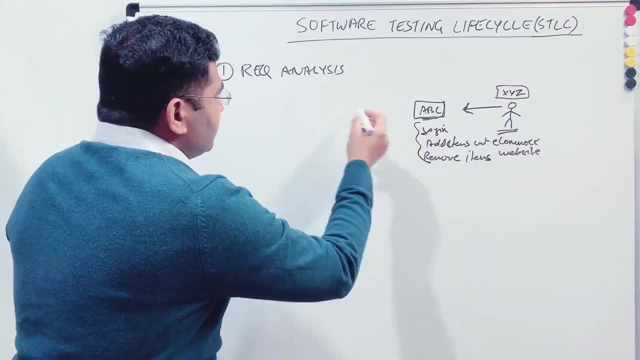 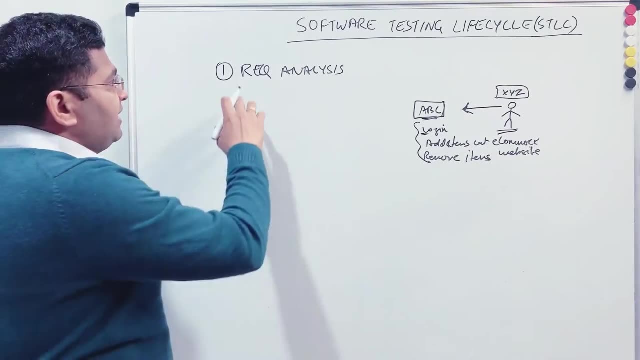 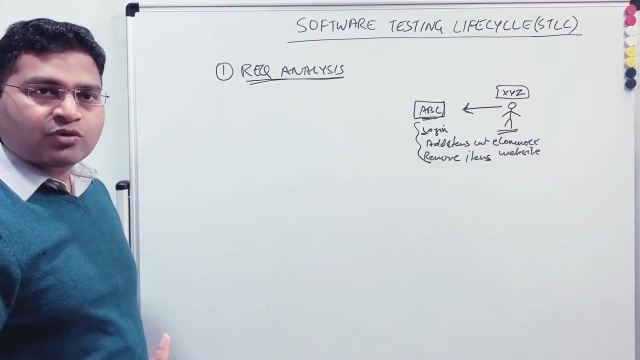 requirements: Okay, These requirements you understand and you analyze those requirements. Okay, You analyze what, all possibilities, what all test cases will be there And that all analysis happens into the requirement analysis phase. So, basically, testing team understands the requirement, If there are any. 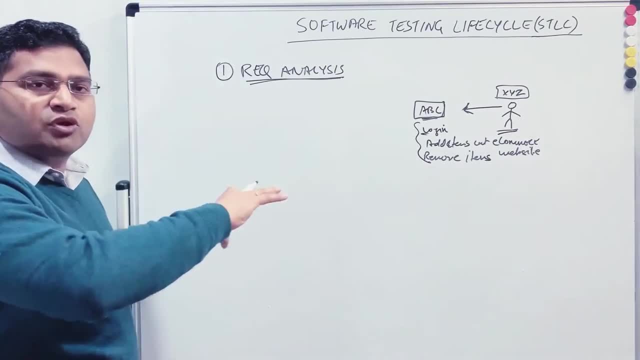 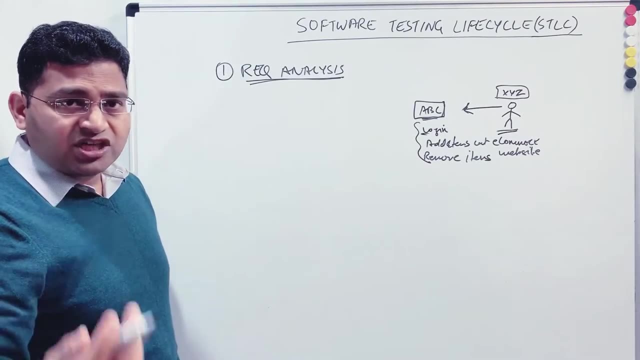 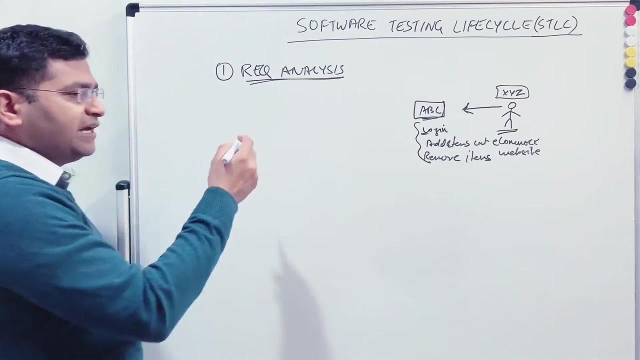 gaps. they provide the feedback to the requirements team or the development team or product owner in current case. So if if say, for example, you are working in a agile development approach, then you will get the requirement in the form of user stories, So you will analyze those And, based on 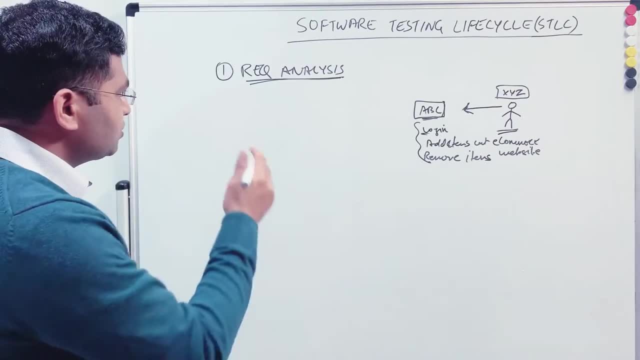 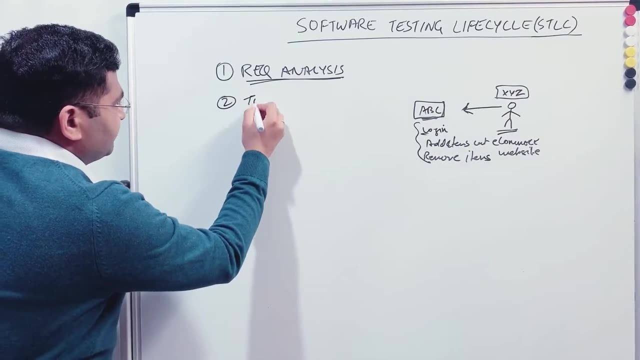 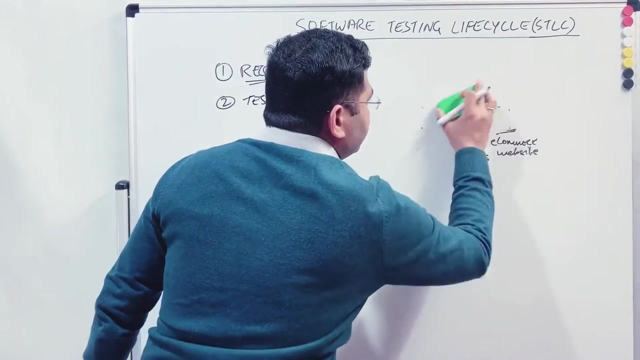 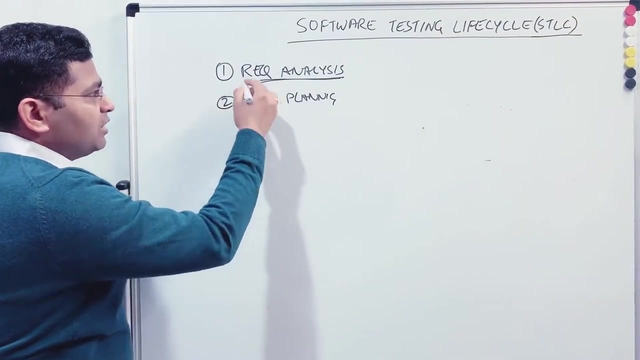 that analysis, you will start your testing work. Okay, So once the analysis is done, the next phase is basically the planning phase. Okay, So test planning. Okay, Let me get rid of it. Okay, So the next phase is test planning. So what happens in test planning? So you have. 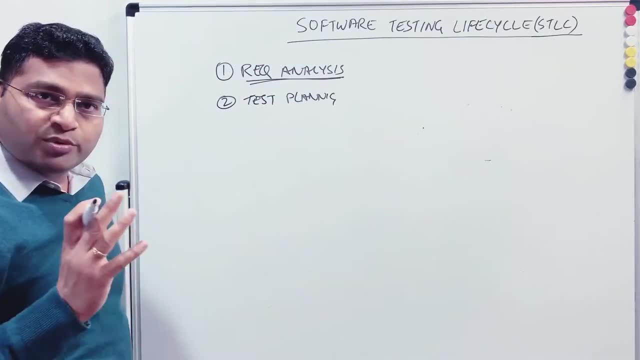 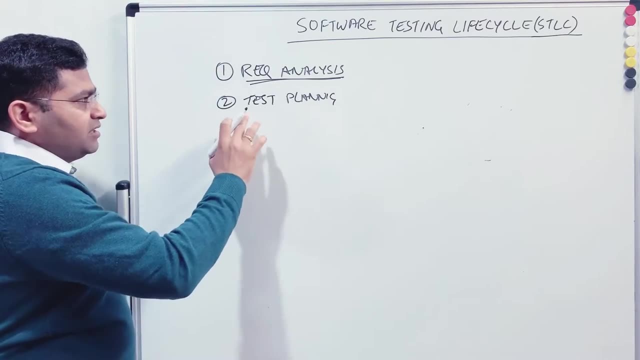 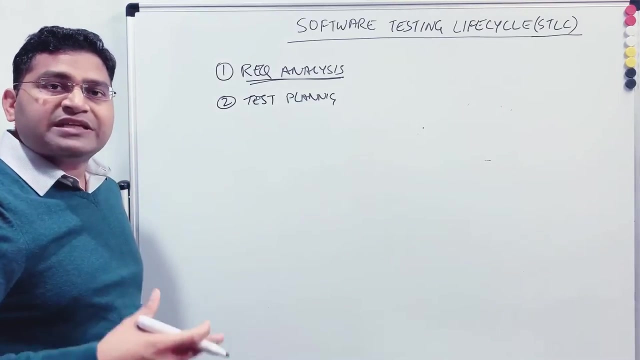 all the requirements and now you understand what all needs to be built and what all requirements are there and how you are going to test right. So once you, as a team or tester, understand the requirement, then you start the planning. Now in the test planning, you start with the test plan. 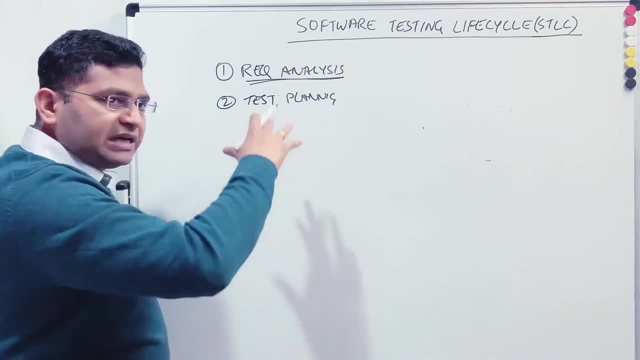 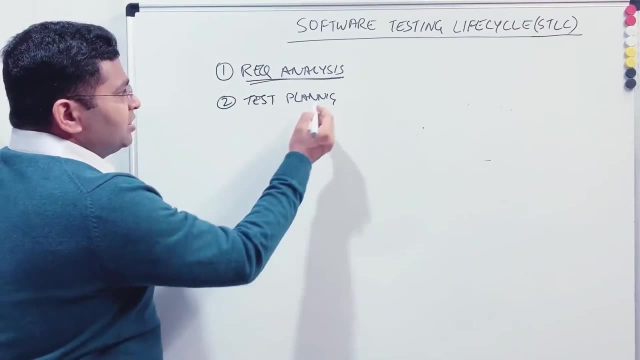 Okay, So if you are working in the waterfall approach, you will write the complete master test plan and then the phase test plan separately. But if it is, you know, agile, then in that case you will still do planning in each iteration or each sprint. right, You will write a quick plan. 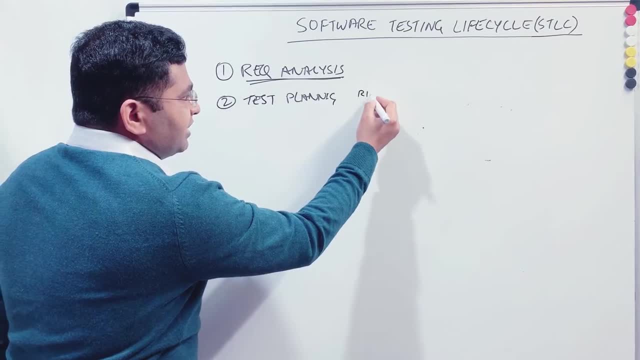 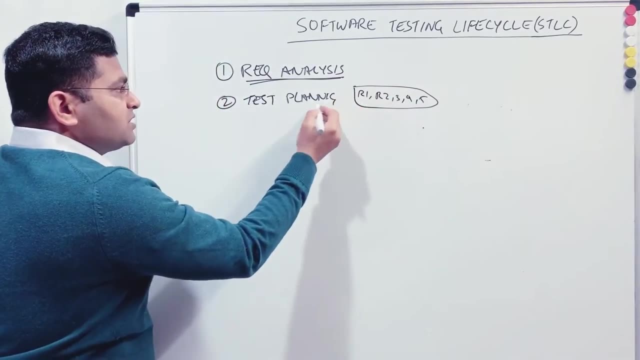 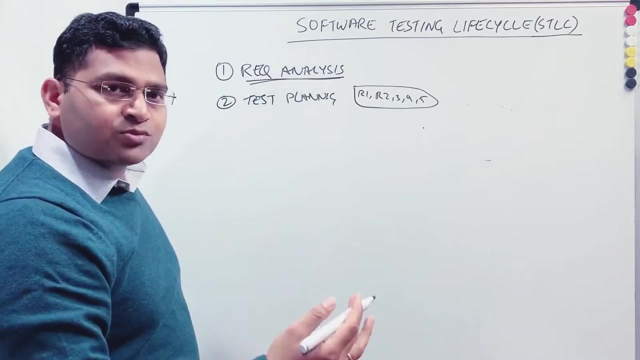 for whatever requirements. for example, you have taken requirement one, two, three, four, five in one sprint. Okay, Then, for all these requirements, you will start the plan, You will do some little bit of planning how you are going to test these requirements. Who is going to test what will be? 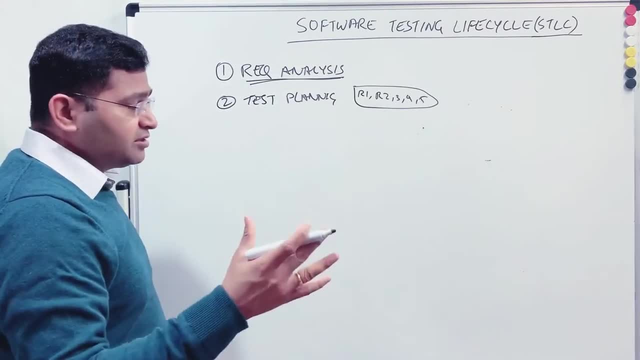 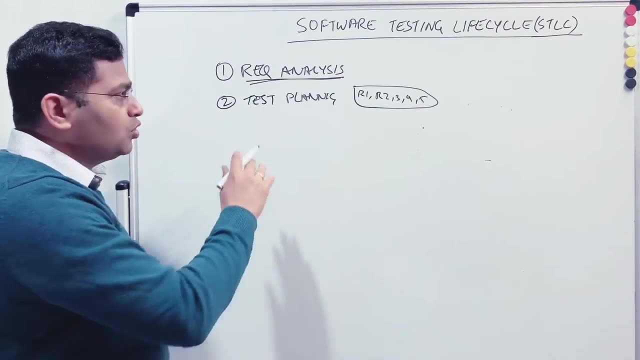 the, you know, like the timeline. So in terms of timeline it's anyways two weeks in sprint, But if you are like waterfall, then you put all those details into your test plan, right. So what is the scope, What is out of scope, What is entry, exit criteria? So all these details go into the 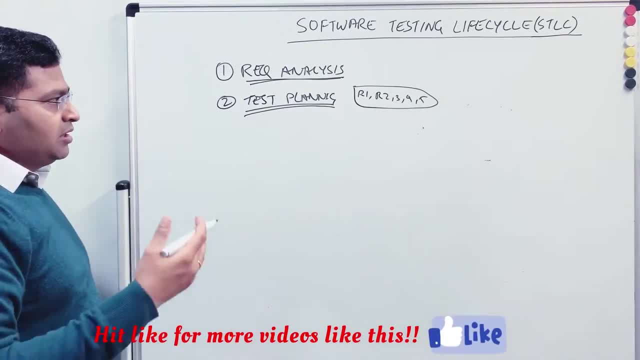 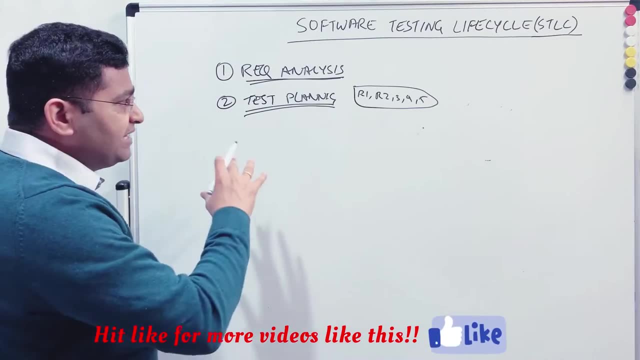 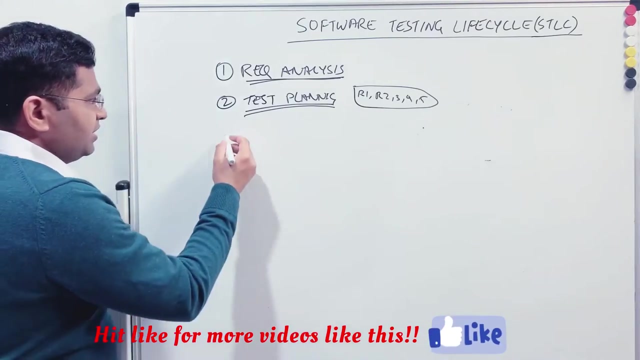 test planning. When you do test planning, you write the test plan right. Um, in agile it is not that lengthy test plan, but still you need to do a fair bit of planning before you can actually start testing the user stories that you pick into the sprints. Okay, The third phase is. 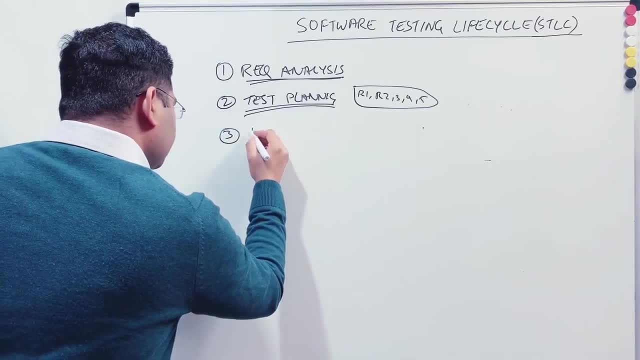 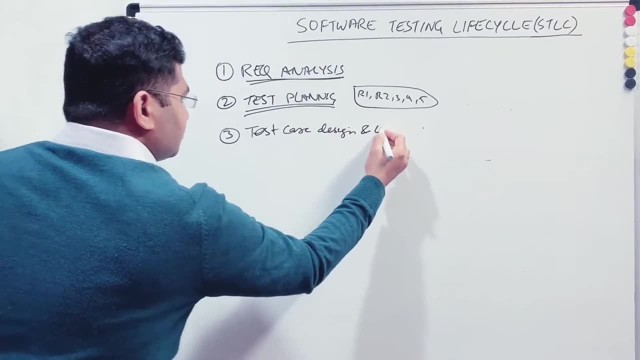 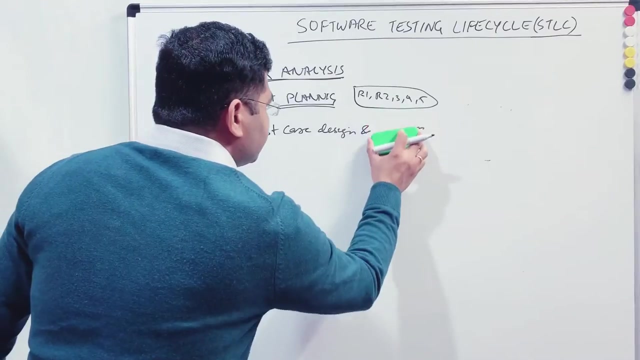 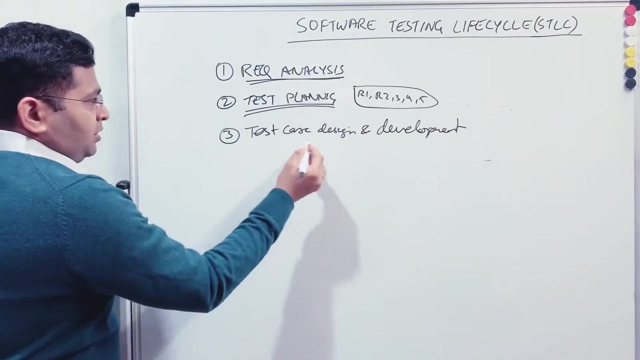 the test preparation, Okay. Or test development, So test case design and creation, Okay. So what you do is basically, or I'll say test case design and development, development, Okay, So you develop your test cases. So when you say test case design, so you apply all the tests you know. 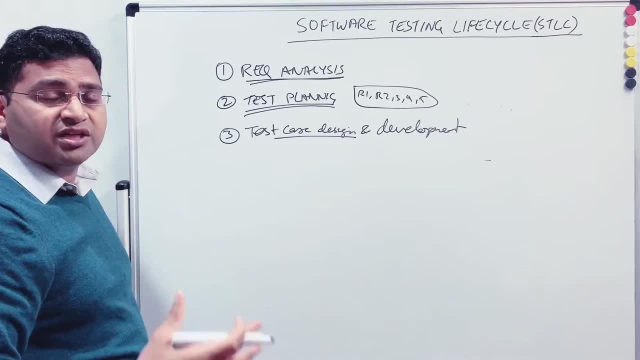 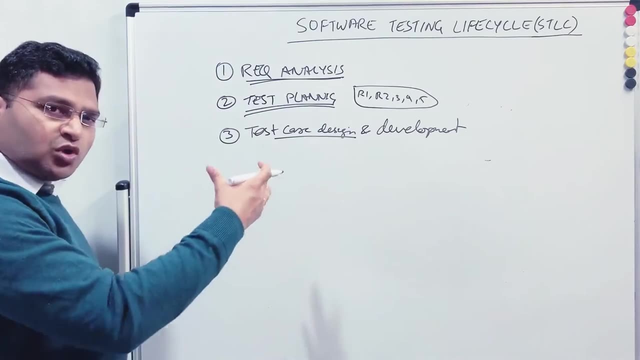 test design techniques. right? So equivalence, partitioning, boundary value analysis, which I'll explain in upcoming tutorials, Uh, so you'll apply all those techniques to design your test cases, what all test cases need to be, you know, added for the functionality, And then you. 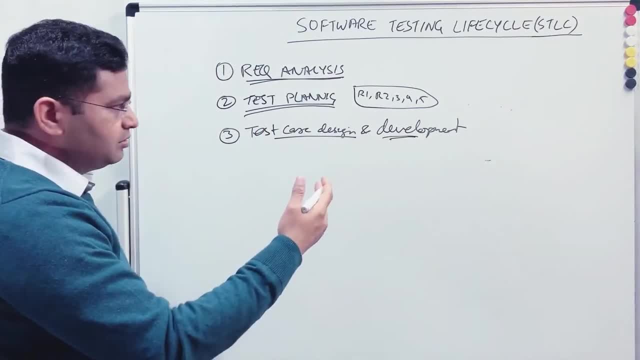 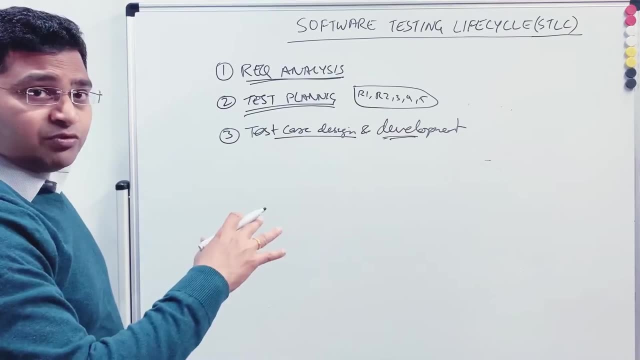 develop those test cases. You write those test cases into the test management tool So you categorize those into different. you know um feature wise, uh, or the requirement wise. you make those test cases and develop those test cases right. 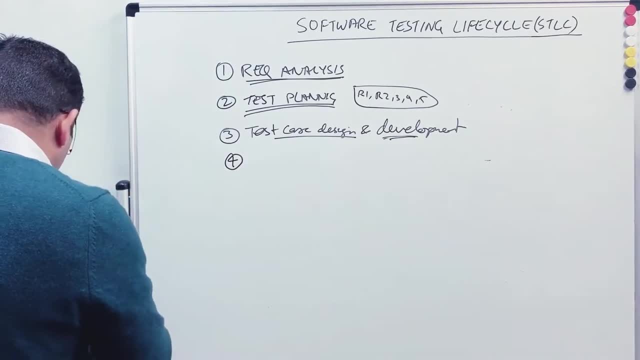 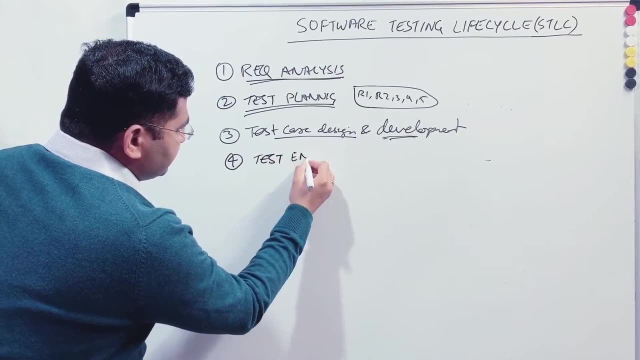 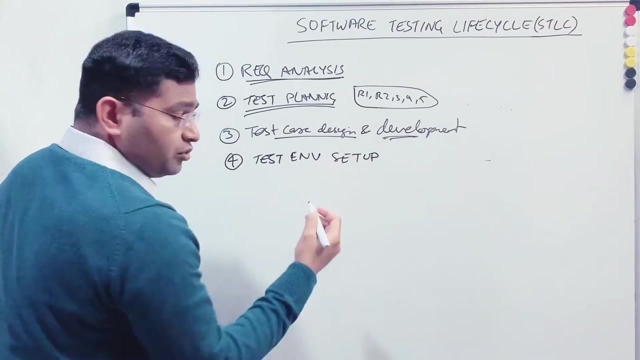 So that's the third phase. The next phase is around, uh, the enrollment setup. Okay, So once you are, your test cases are ready, So you have this test enrollment setup. So usually, if your team testing team has the capability to set up the test enrollment, 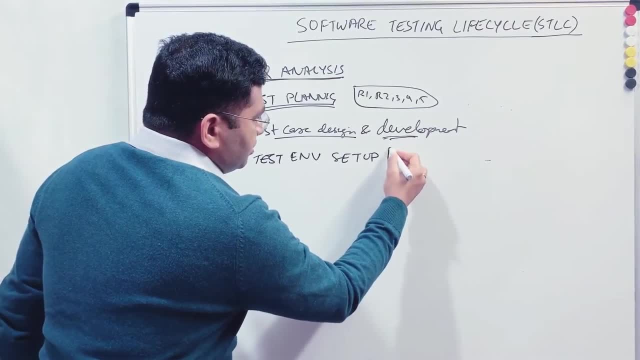 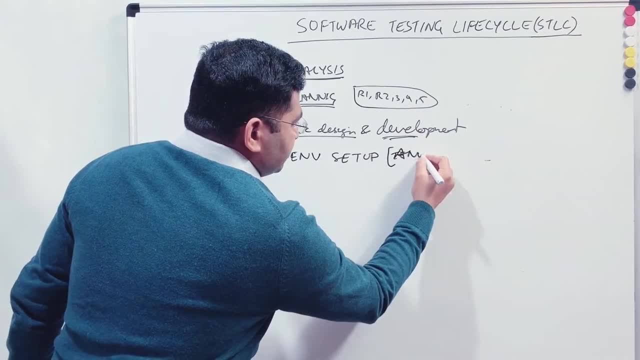 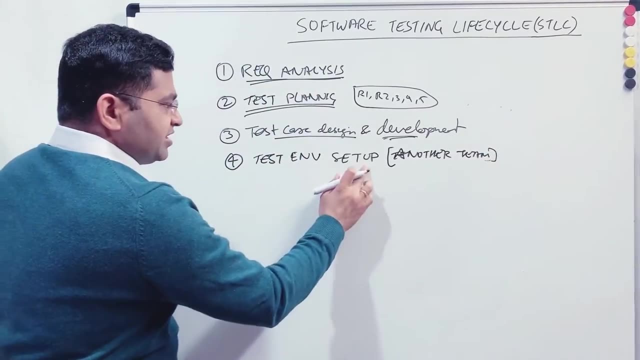 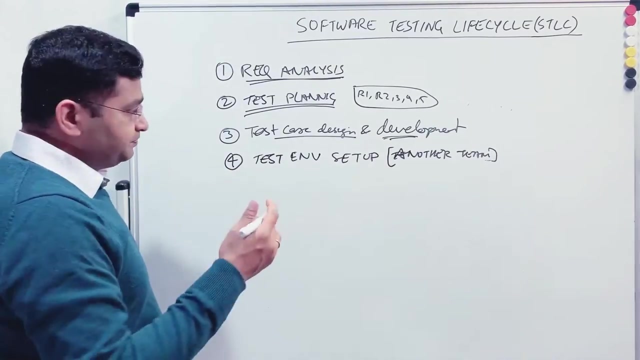 for example, if you are, you know, um, I'll say another team. So you say, for example, your application is really complex, one which requires a lot of integration. usually in banking sector that happens, or telecom. In that case there will. 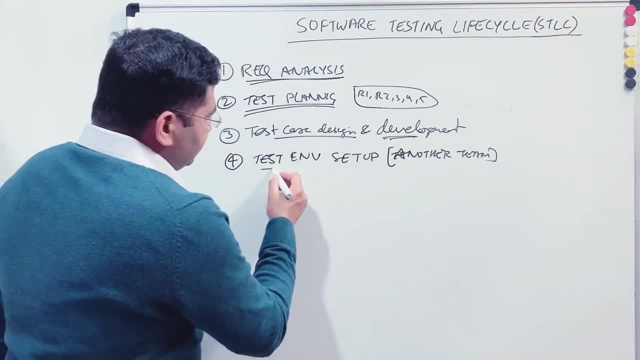 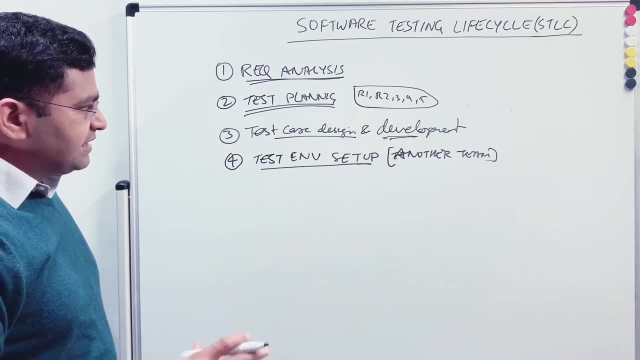 be a separate team which will maintain the test enrollment for you And in the test enrollment setup all the test enrollment related detail or or test enrollment will be- you know, uh- ready And made available to the testing team. And then you have to basically ensure your test data and 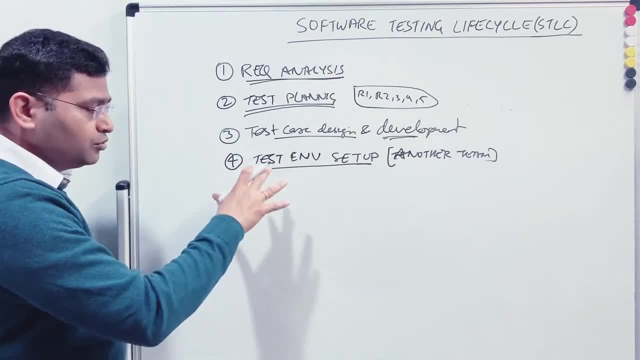 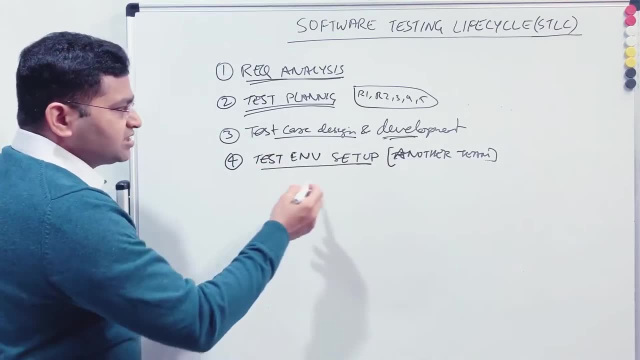 everything is set up there. So test data preparation you have to do and provide to the separate team. or if your team is capable or testing team is capable to manage the test enrollment, test data, they can do the whole enrollment setup themselves. but test data 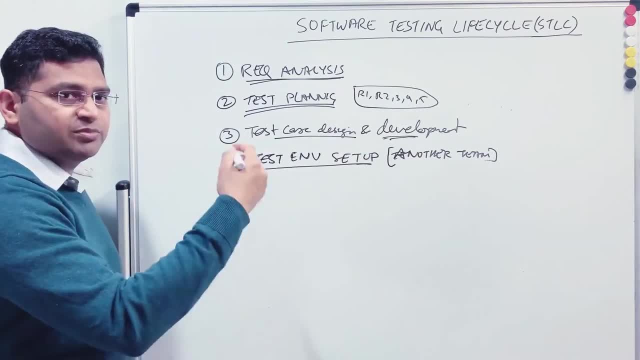 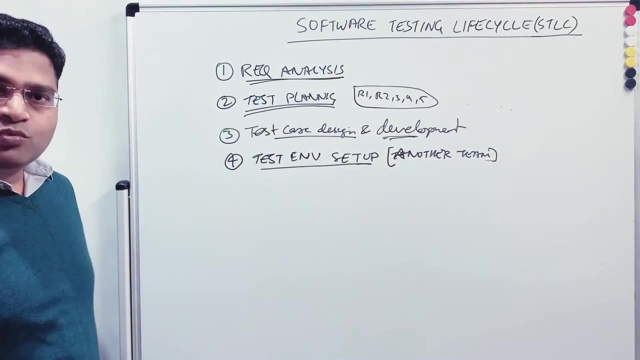 you have to provide to the team if the testing enrollment is being managed by other team, Right? So this fourth is basically test environment setup, because test environment is required for any of the testing that you need to do, right, where you will execute your test cases that you have written here. 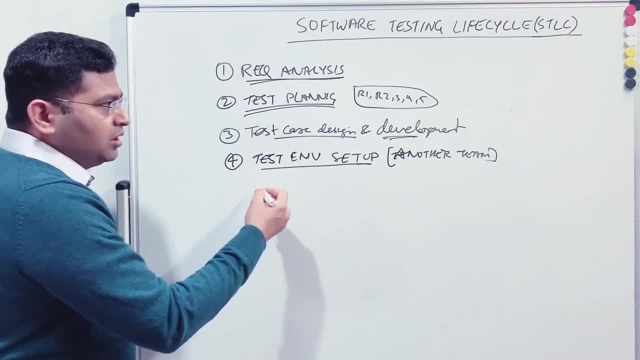 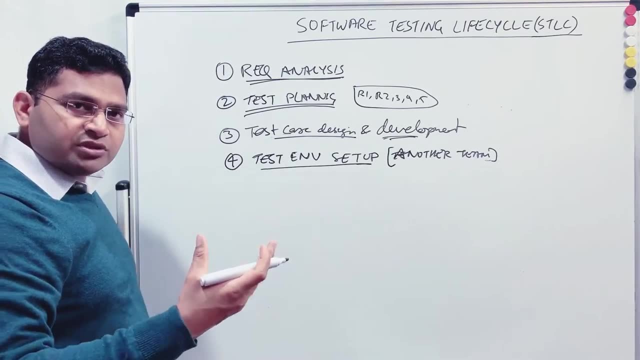 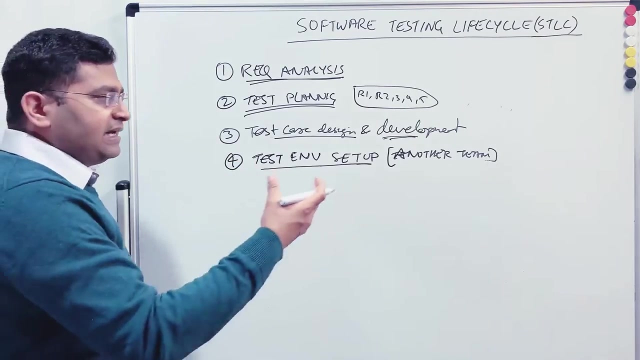 so, once the test cases have been written, you will have the environment where you, where you will have this e-commerce, say, for example, e-commerce website code deployed and then when you launch the website in the browser, in the test environment, it will be visible and then you can verify the website look and feel, adding items. so all the features that are. 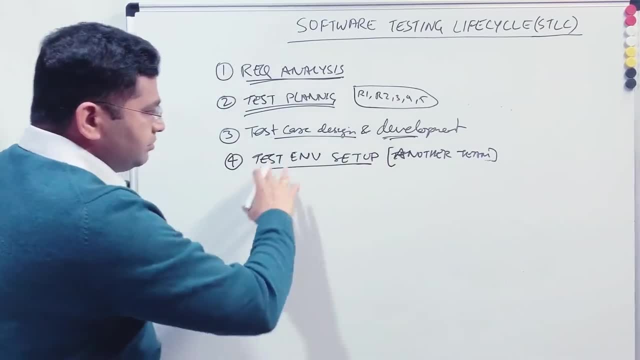 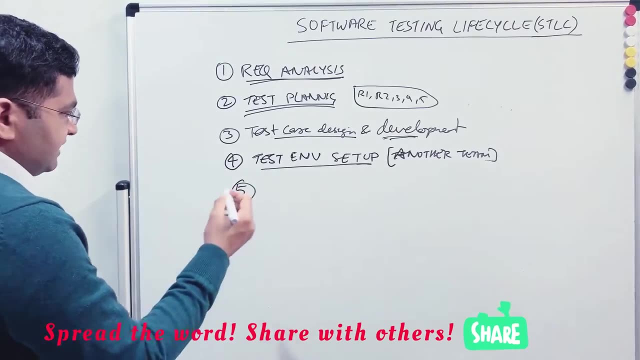 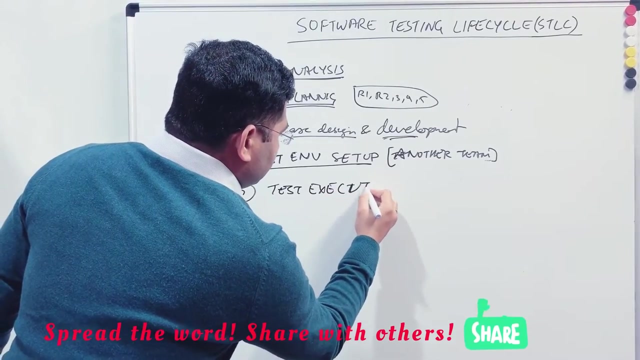 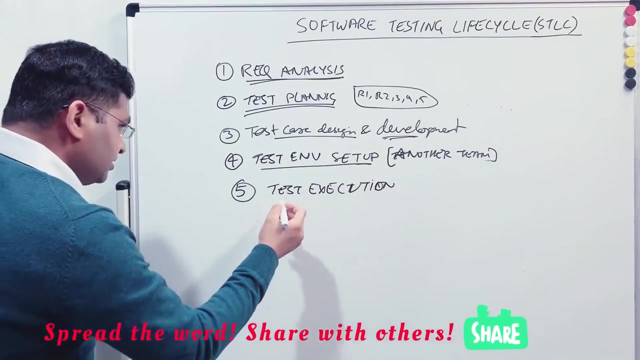 available there in that particular release, you can start, you know testing that. so test environment setup is necessary. so that's the fourth step. fifth step is test execution. all right, so once the environment is ready and you have test cases ready, right. so the next step is the test execution. 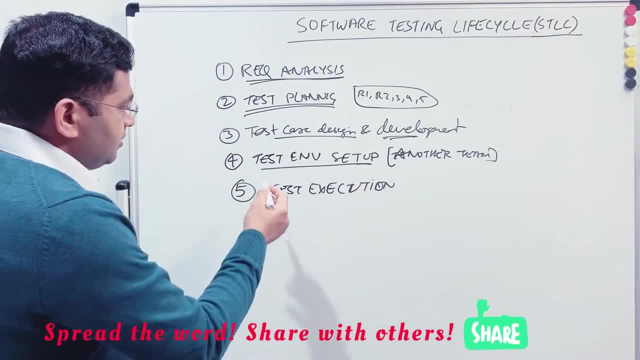 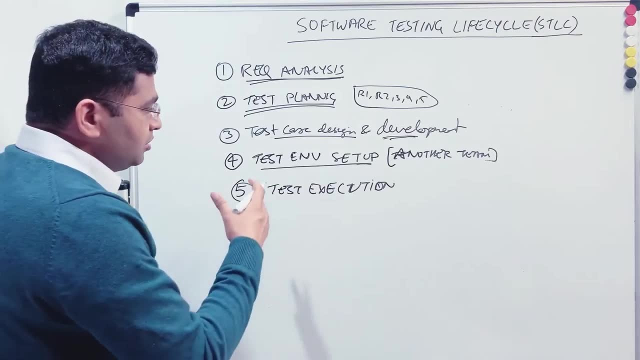 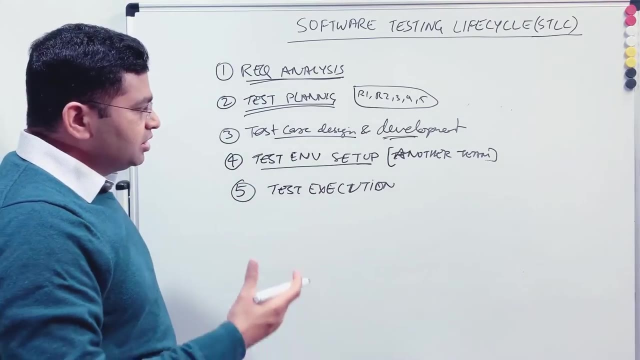 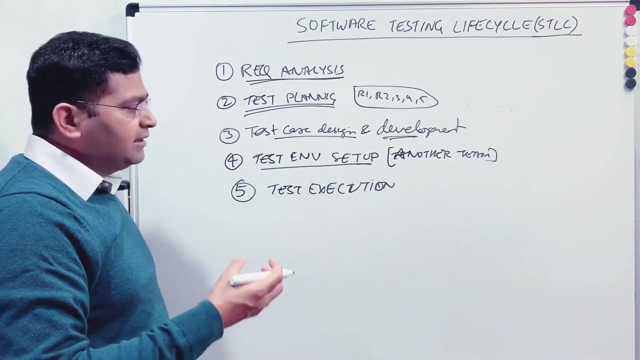 so how will you verify that the test cases that you have developed very far meet or pass or fail, right, so those that happens only when you will execute. so when you execute your test cases, you verify that the website is being launched. okay, so you open the browser, you launch the website. 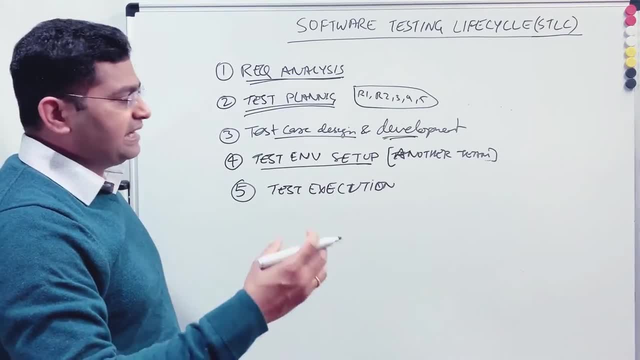 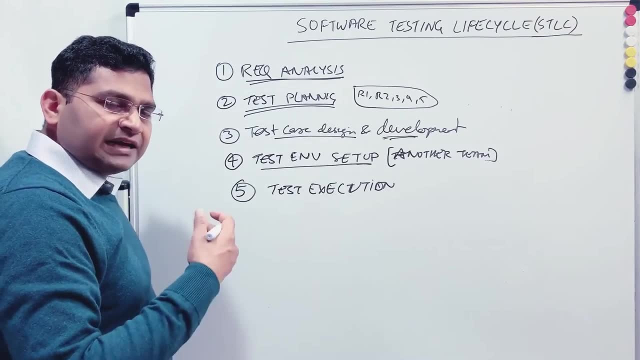 and then you add the item to the cart. if the item is getting added, the test case is passed. so, for example, you have a test case for adding item into the card. the item you remove gets removed successfully, that test case is passed. if any of these you know, 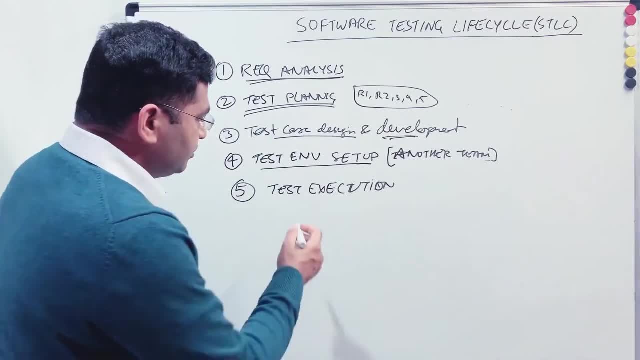 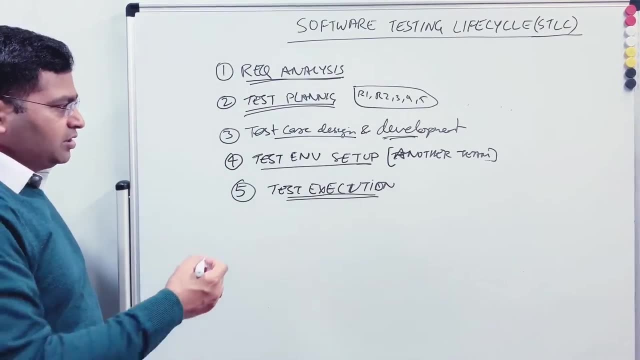 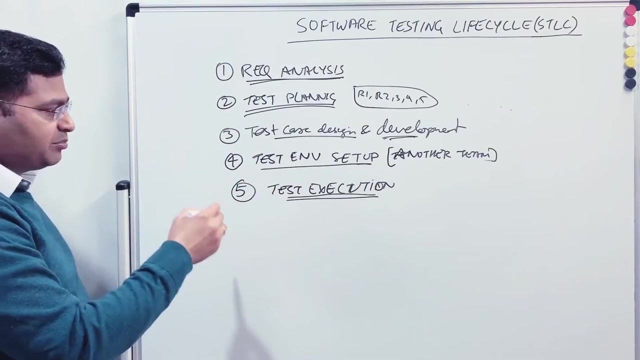 operations fail, then the test case fail, right. so in the test execution you execute the test case and then verify whether the test case got passed or failed. so that's the another phase of software testing lifecycle. so these are step-by-step phases that happen into the software testing. 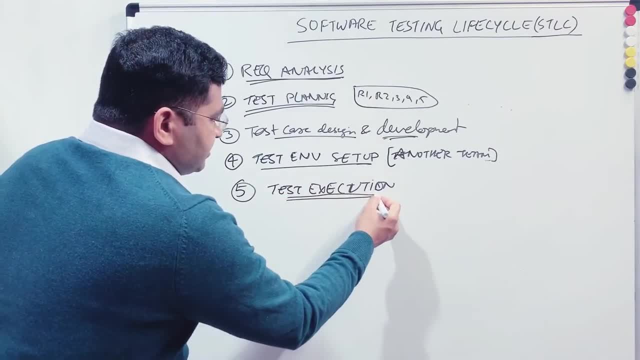 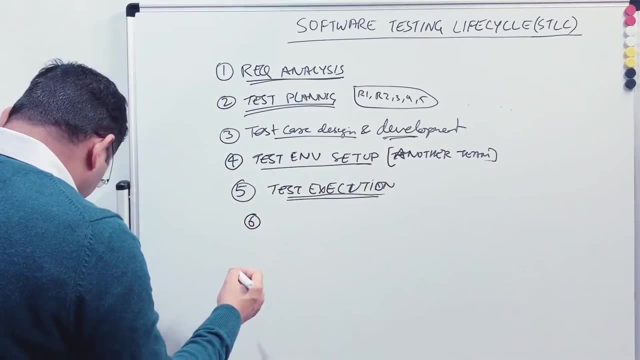 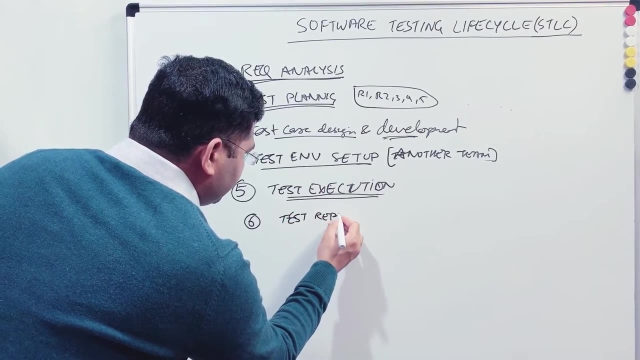 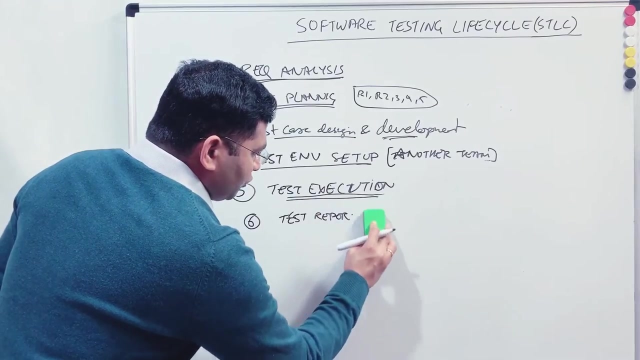 lifecycle or stlc. so after test execution has been completed, right. so after test execution has been completed, the next phase is the exit criteria and reporting. so basically test reporting. you can say test reports okay, or test reporting. so in test reporting what you do is once your 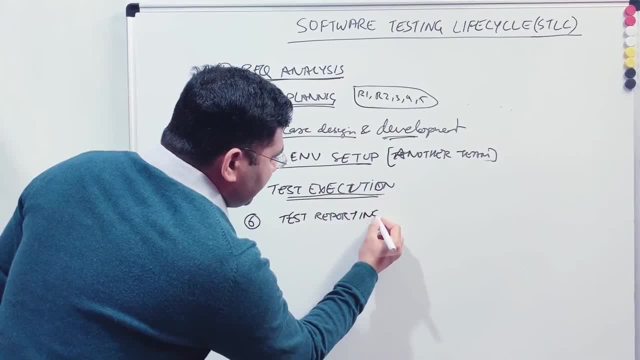 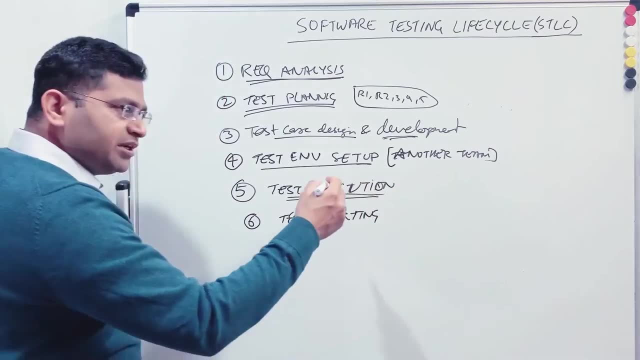 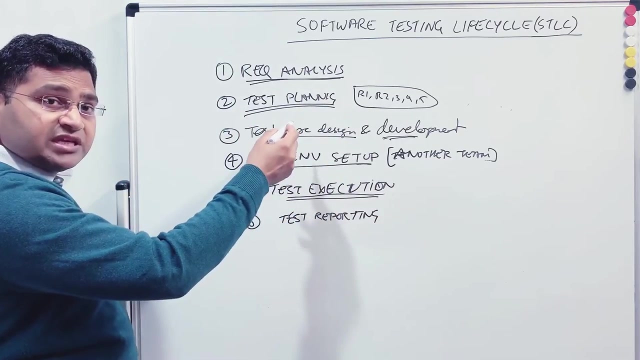 test cases or all the testing that has been planned has been completed, you need to provide the report right so say, for example, execution happened. if there were test cases that failed, then those test cases will be reassigned to the developer, or basically, the defects will be assigned to the developer to fix. they will come back to you to the testing, to. 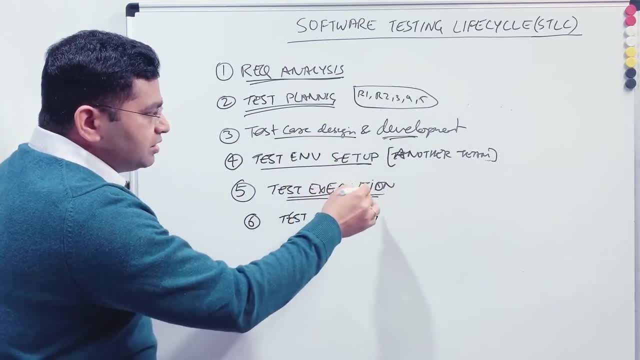 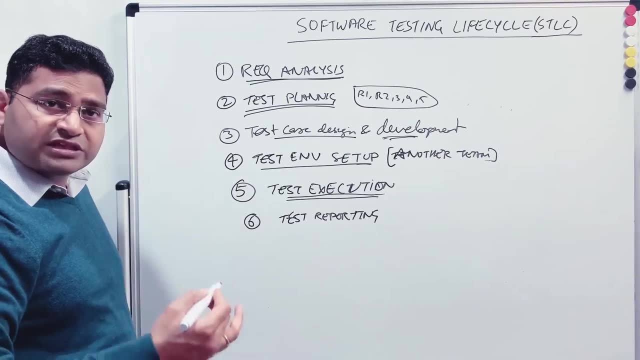 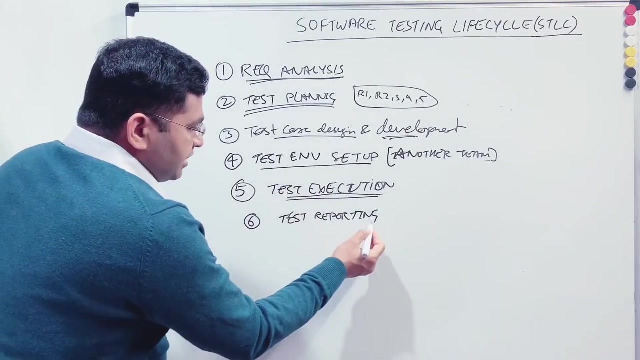 verify again. and once all the testing has been passed, then you provide the report. or even if there are open defects and those defects are accepted by the relevant stakeholders, then you and they say, yes, these defects we will fix in next release. then you start preparing the test report. 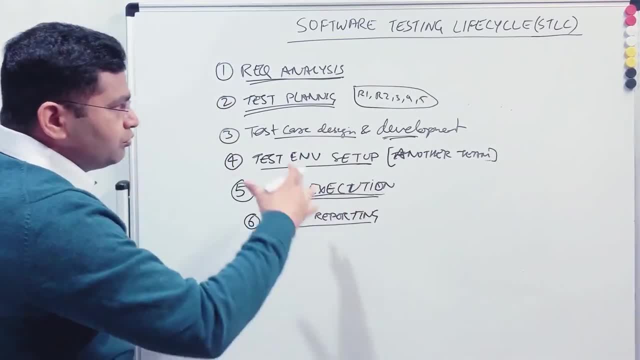 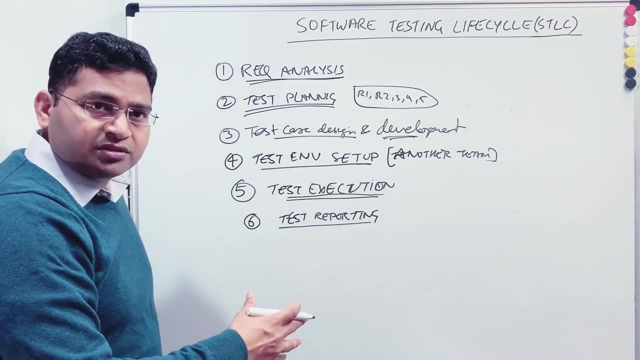 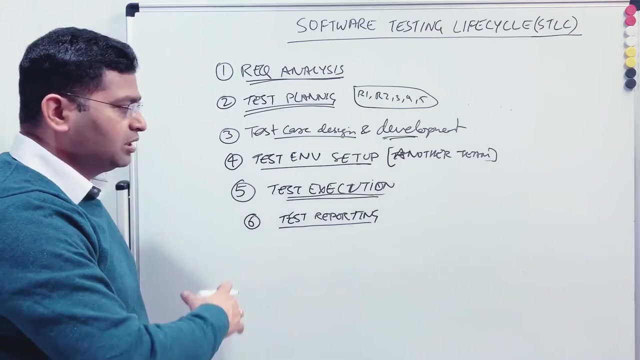 and what you prepare in the report is how overall testing went through, what all testing has been done, what was in scope and what is the overall confidence right. so which will help you to decide, or which will help the team to decide go and no go, whether they need to deploy in production or 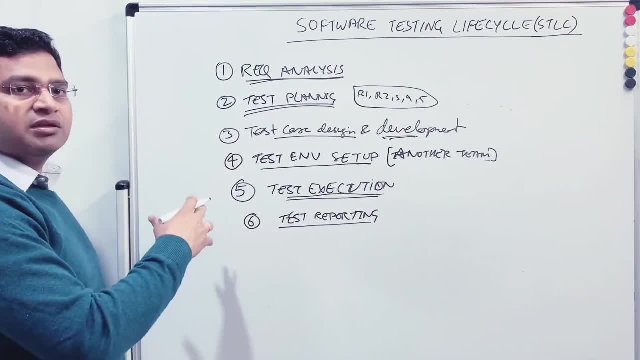 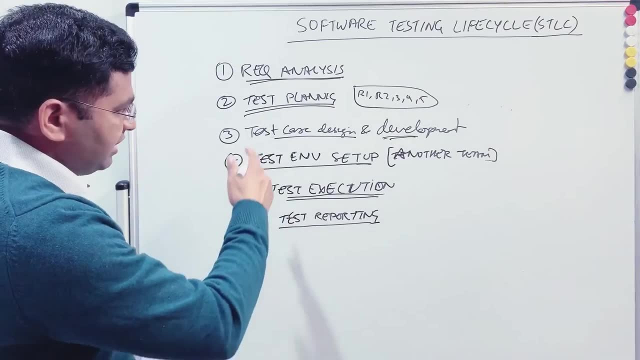 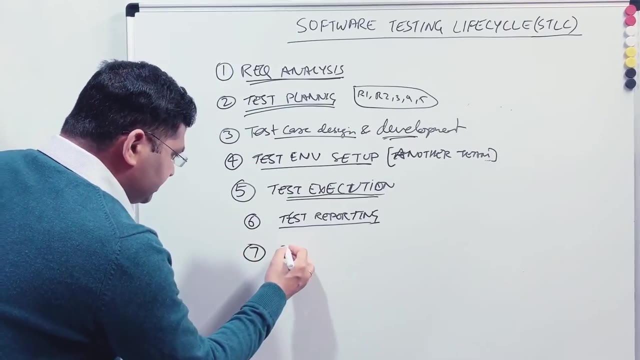 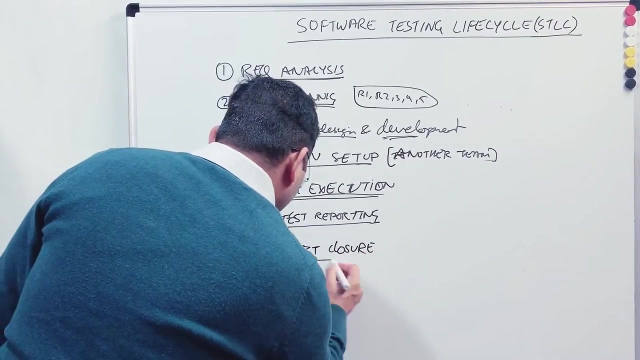 they want, you know, like fix more defects or or make the software more stable, right? so test reporting, um is the reports that you produce after the testing has been done, right? and then the seventh phase is around the test closure. okay, test closure, so test closure. what you do is in test closure now, after the overall testing has been completed. 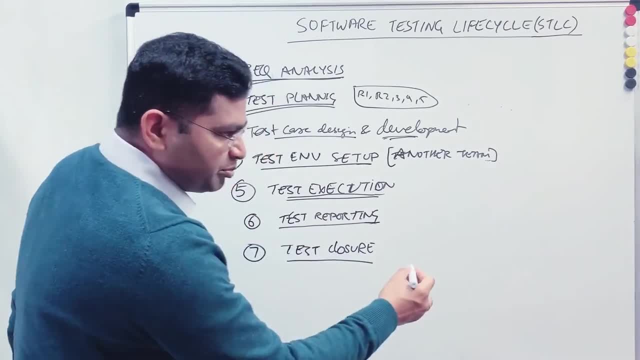 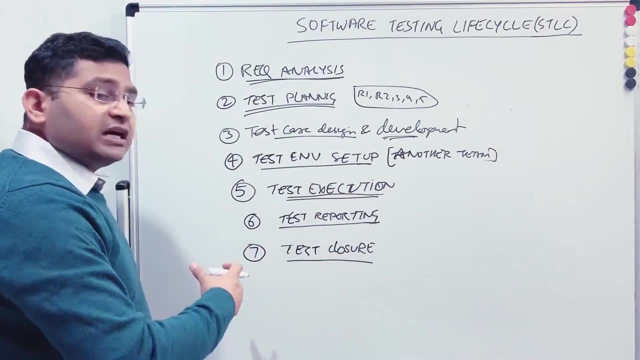 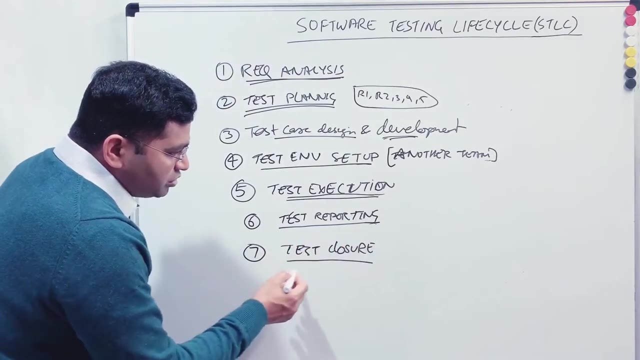 and the you know software has been deployed in production. so in test closure activities what you do is you produce all the documents that are helpful for other teammates. so for example, there is another team who is maintaining that particular software in production. then in the closer documentation you have all the documentation around the test cases where 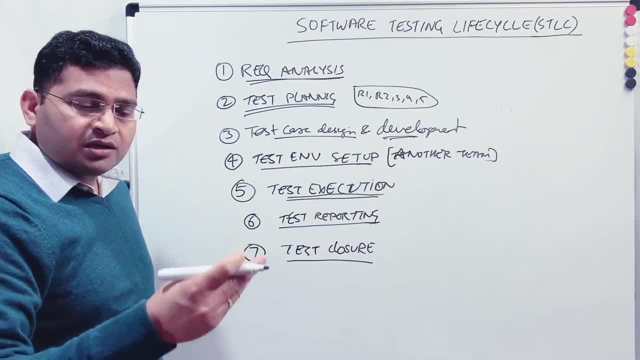 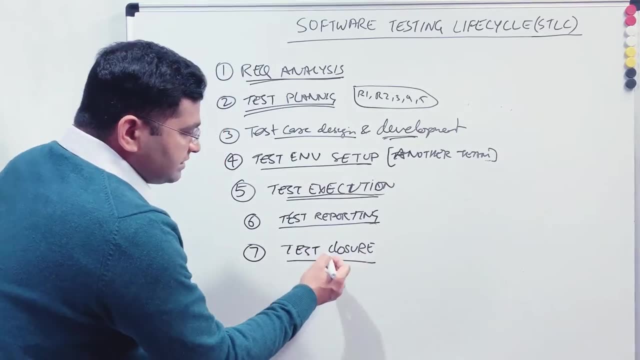 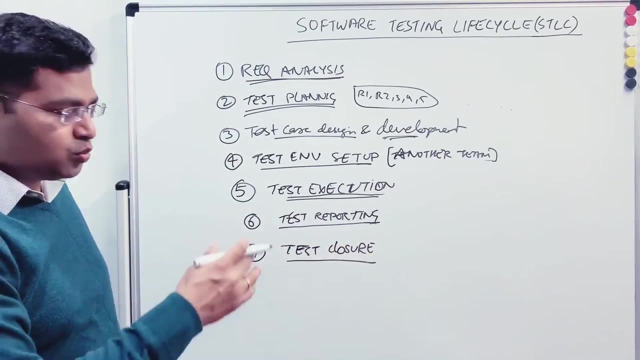 the test cases are what testing has been done, what all artifacts have been produced in terms of test plan, summary reports, etc. all those details, along with the development document, need to be, you know, produced for the test closure activity, so once the complete testing has been completed, or 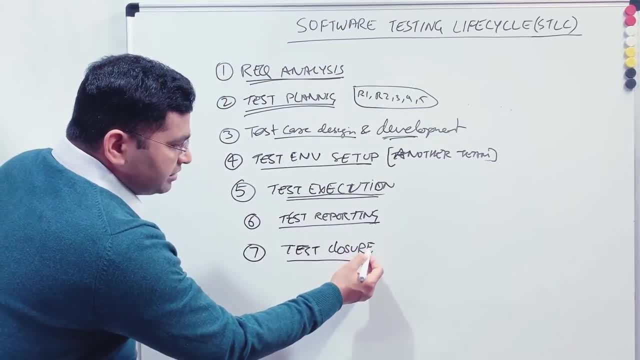 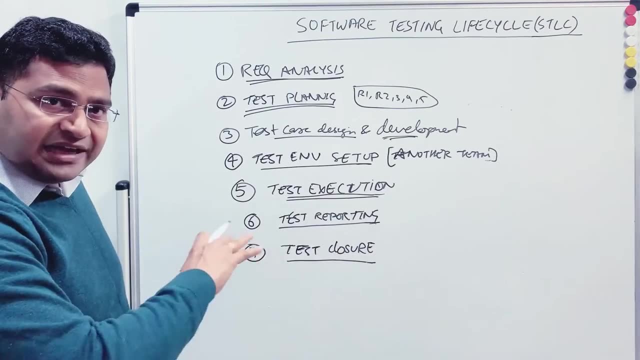 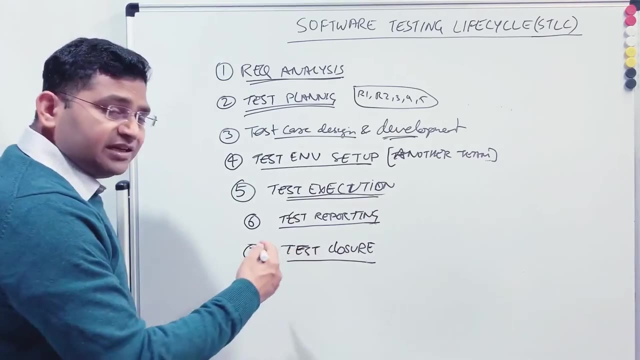 the overall testing for the project has been completed, you provide the test closure summary report or the test closure documentation. okay, so all the test closure phase has the activities- different activities- and depending on which type of software you're testing based on the context, you have to provide the relevant documentation for that, okay. 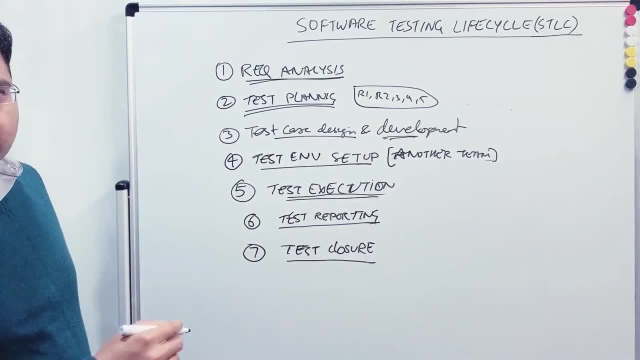 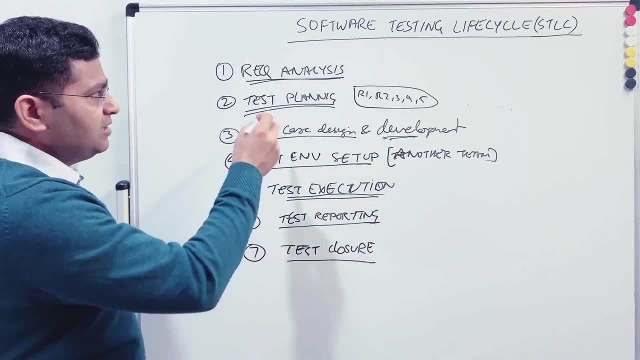 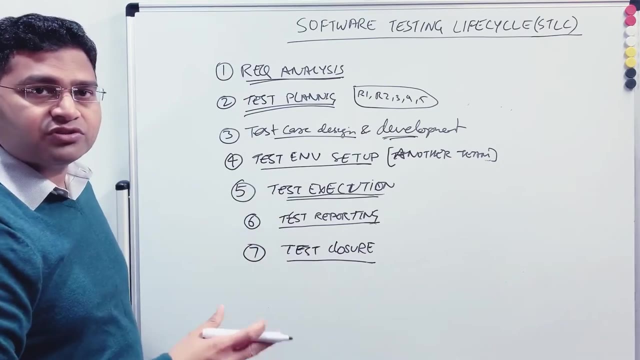 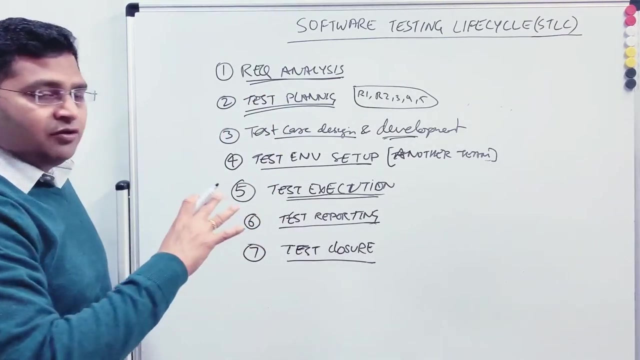 now, these are the seven phases in software testing life cycle. right, so this is the process of software testing life cycle, which you need to understand, and understand very clearly for interview purposes and even for working in any of the software testing project. now, this stlc remains same for the waterfall or agile, it doesn't matter, the only difference. 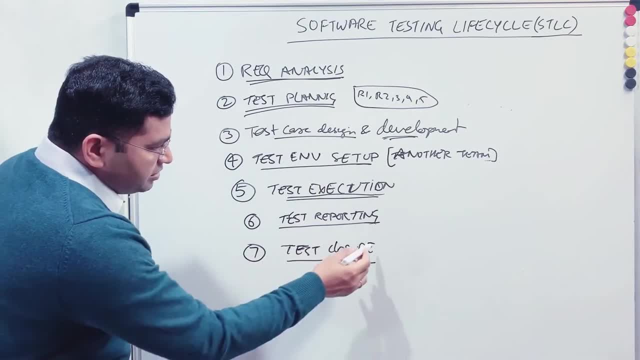 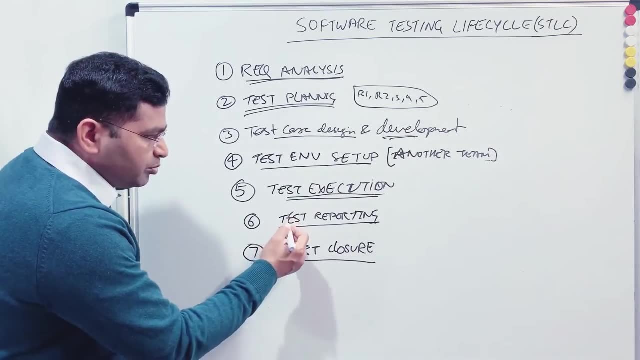 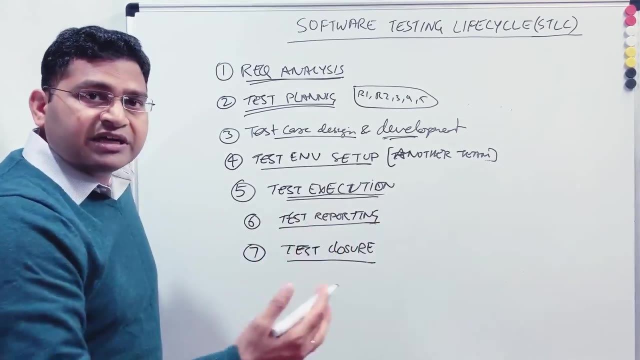 between the two is that you have to provide the test closure report for each sprint. so the test closure report basically happens is, you know, in the closure activities you do not provide closure reports in agile for every sprint. okay, you do have the reports, but those reports are automated out of the tool. say, for example, if you are using jira, they are out of the jira itself. 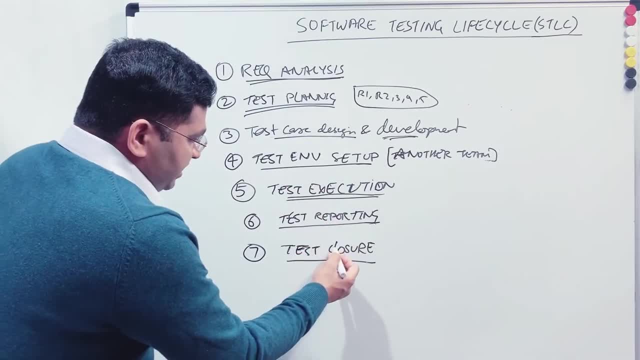 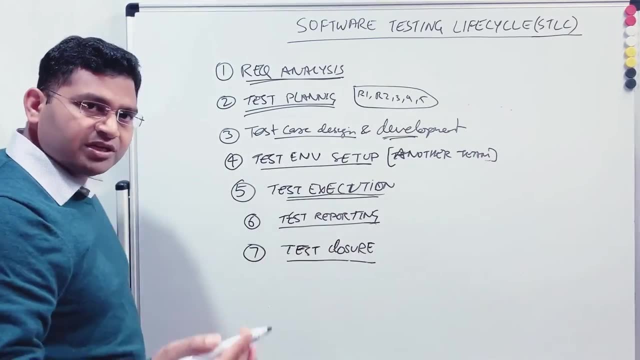 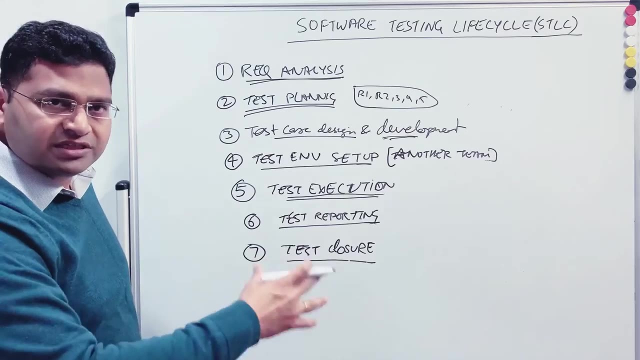 you have the gadgets and you can pull the reports of the execution for each sprint. um, you know automatically in jira, but in agile the test closure report will happen every sprint, right. so which is basically similar what we do in the waterfall approach. the only difference is in the terms of timeline. in waterfall project might run for a year, but agile 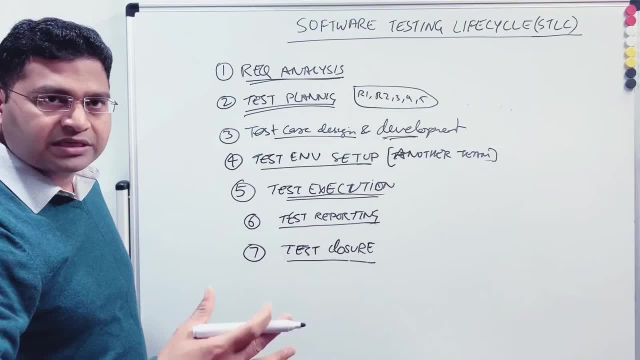 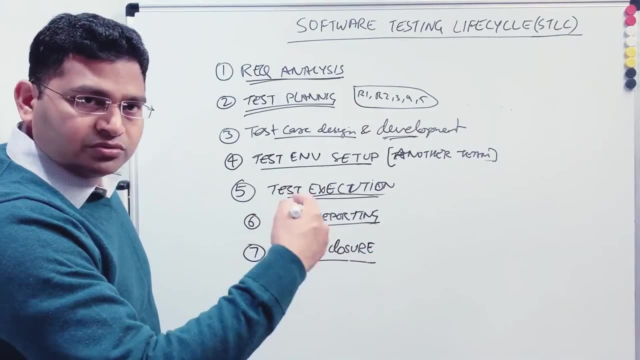 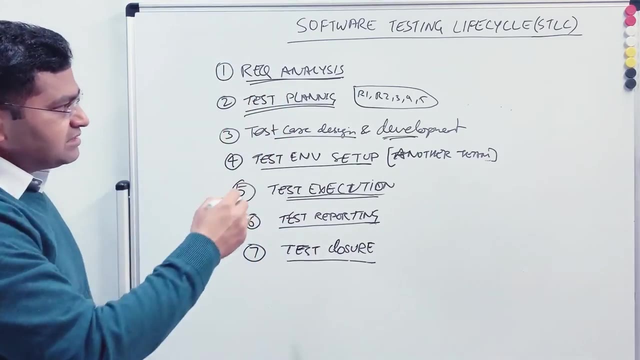 usually the delivery happens every month or you know every three months at the max. so you have to provide disclosure. you know reports or activities after every. you know three months in agile or after every month. right, it's as per the organization's requirement, but in terms of phases, 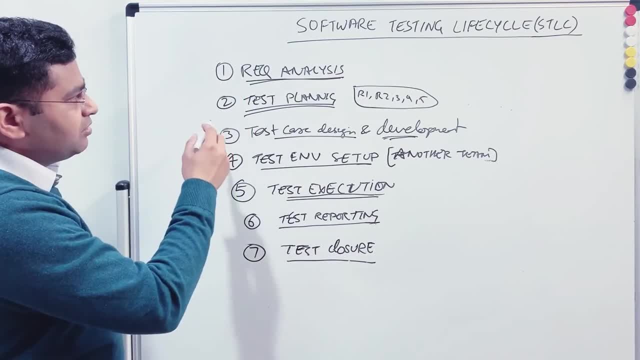 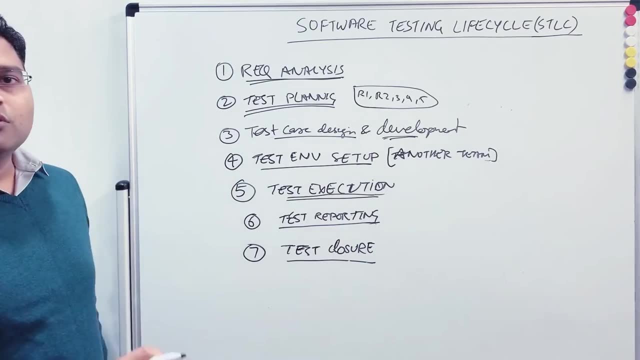 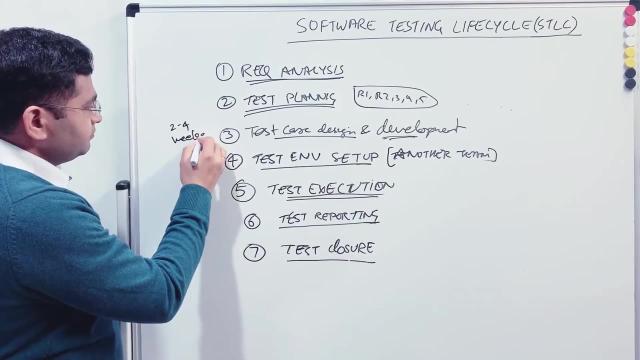 you have to follow. you know similar uh phases or the test activities in software testing life cycle. it doesn't matter. you are working in v model, waterfall model or agile scrum approaches right. so if you are working in two weeks two to four weeks scrum in agile, you will do. you will do. user story.